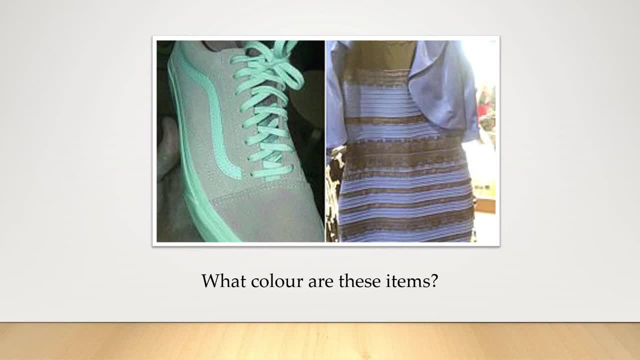 full range of colors in the first place, or that you don't have vision impairment, or that you're from a culture where you even recognize that this is a shoe and that this is a dress. We're all looking at the same objects, but how we interpret it depends on so many things. Three main categories: 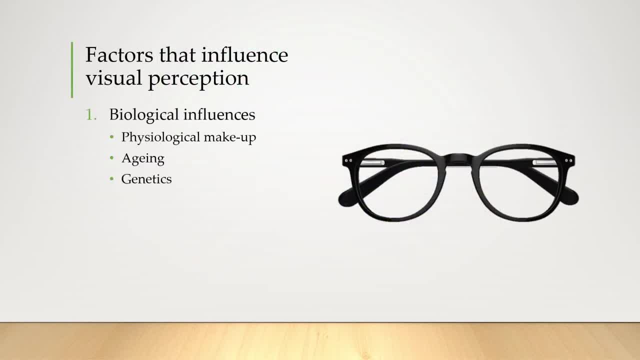 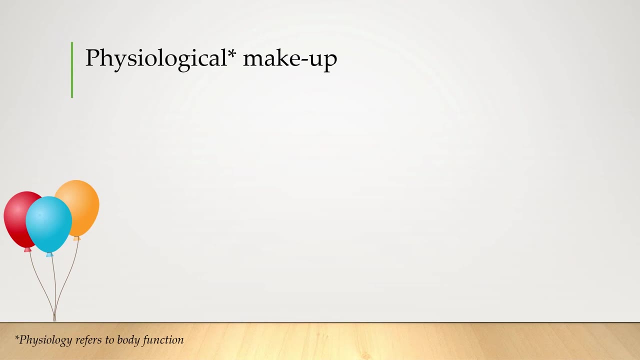 of factors that affect how we perceive vision are biological influences, psychological influences and social influences. We're going to spend a lesson on each of these things. starting with biological influences, Let's have a look at how physiological makeup affects vision. Well, since the thing that helps us see is our visual system, if any part of it is damaged or 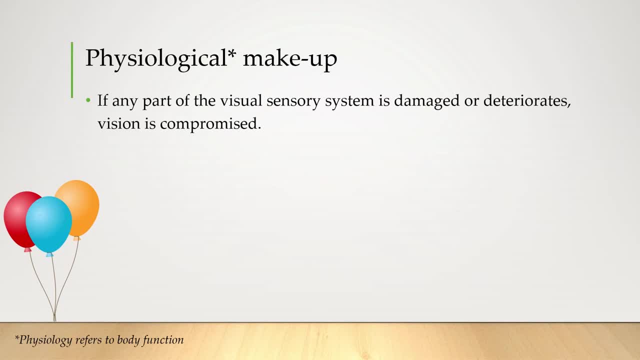 deteriorates, vision will be compromised. One example is achromatopsia, a condition in which you might have partial or a total absence of color vision. Now, this is different from colorblindness, which is where people have difficulty distinguishing between color. but more on that soon. 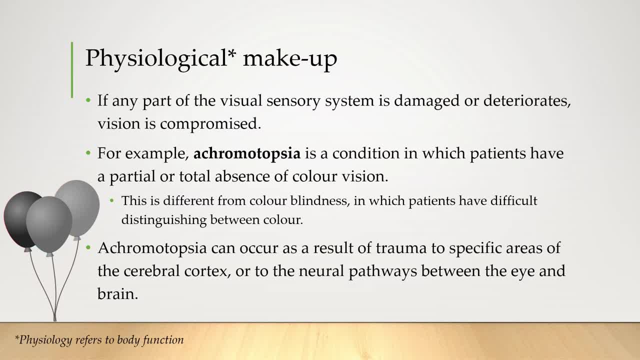 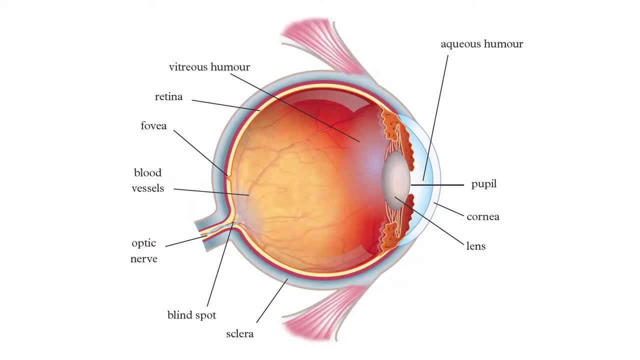 Achromatopsia can occur because of trauma to specific areas of the cortex or to the neural pathways between the eyes. Speaking of the eye, let's have a quick look at it again, even if just to remind ourselves of how complex this organ is- Pretty much any part of the eye can be affected, thus affecting vision as well. 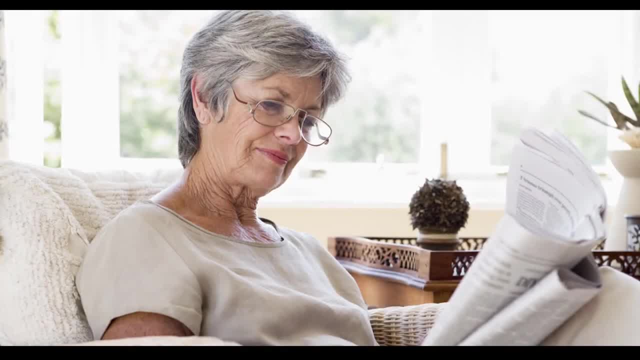 as we'll soon see. One common example of affected vision is with the elderly. Many of you will know older folk who need reading glasses or who might perhaps have had surgery for cataracts. With old age comes wisdom, but unfortunately a lot of other conditions as well. One reason why reading glasses: 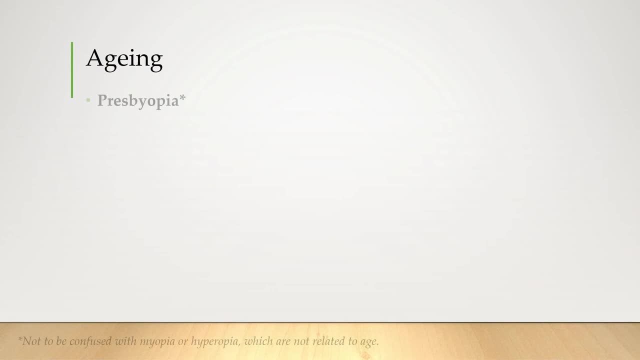 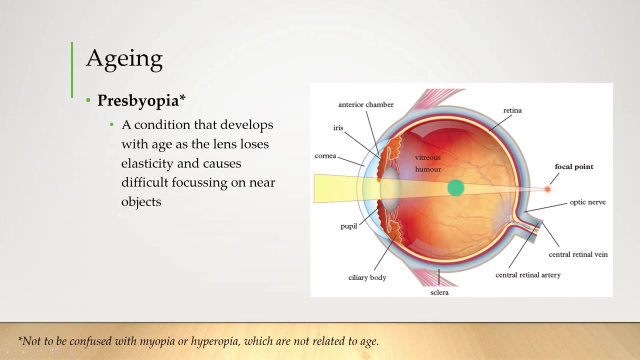 become so common in old age is because of a condition called presbyopia, which is what happens when the lens starts to lose elasticity and isn't able to bend light as effectively anymore, resulting in the person having difficulty focusing on near objects. Although this condition 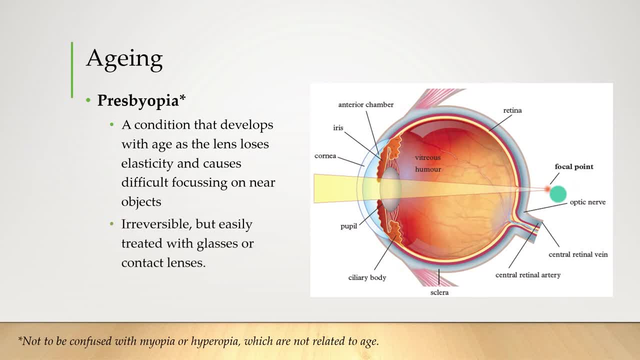 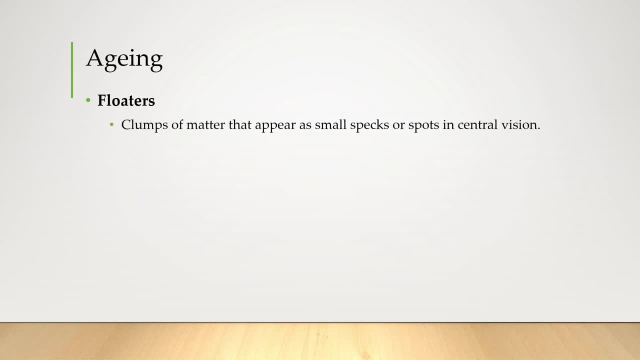 is irreversible. it's easily treated with glasses or contact lenses. Having floaters is another condition that comes with old age, which is when you get clumps of matter that sort of appears like little specks or spots in your vision. And this happens when the vitreous humor, that central sort 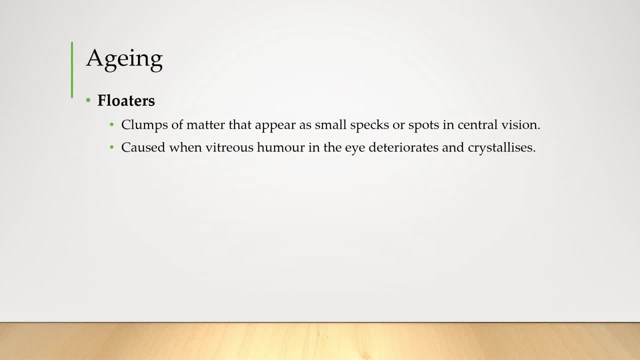 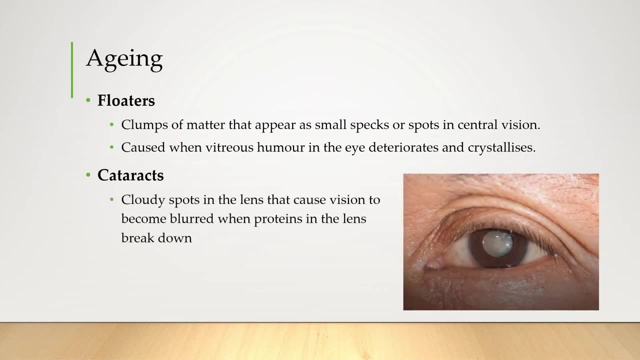 of liquidy part of the eye deteriorates, starts to crystallize. Cataracts is something else that you may have heard of before. This is when you literally see this cloudy spot in the lens. This happens when proteins break down in the lens and it causes vision to become blurred. It naturally occurs with 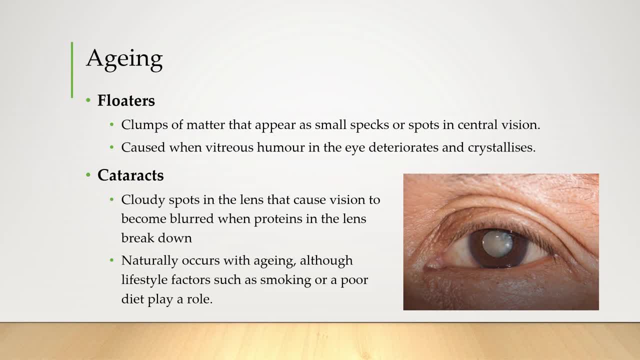 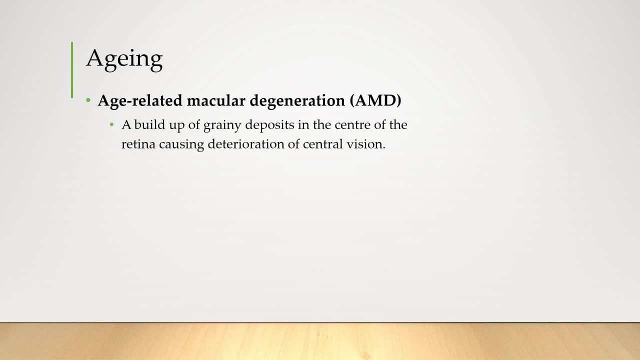 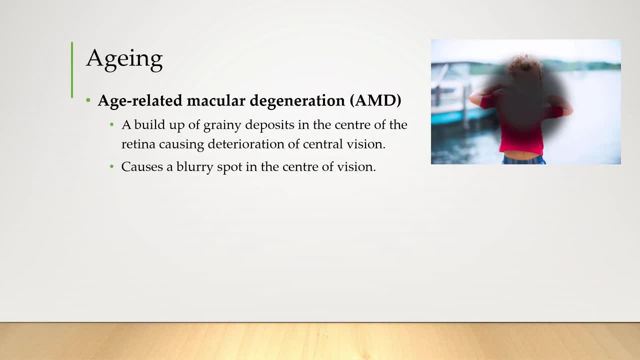 So people with AMD sort of have this problem. So people haveándy been dealing with something along the lines of glaucoma. people with AMD sort of have this problem. So people with AMD sort of have this problem. So people with AMD sort of have this problem. 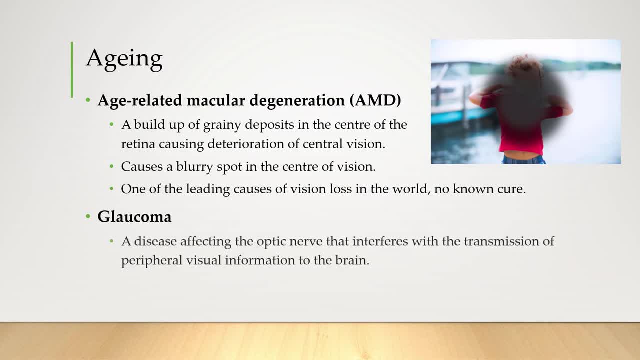 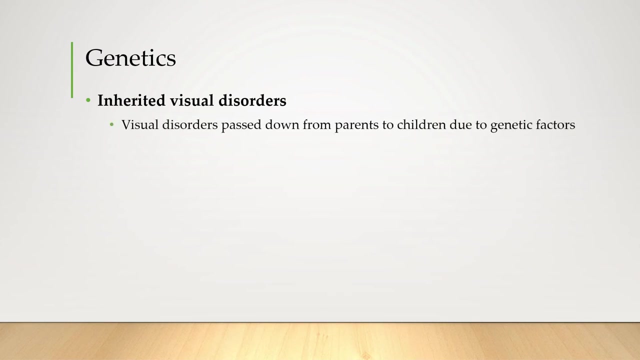 So people have a condition of g. Let me explain why this can basically be described as a disease. This is a type of disease that rightfully, is a part of human life. therefore, it's related to Chi Chi visual disorders, which means conditions that get passed down because of genetic factors. 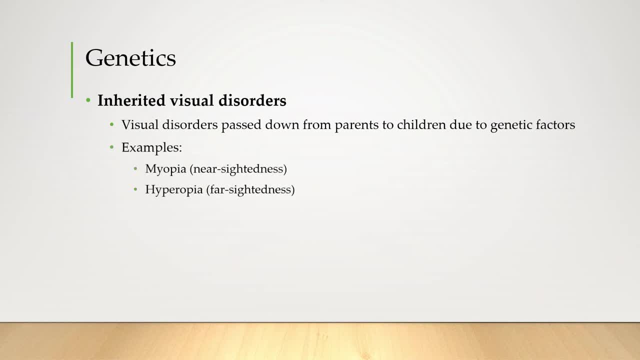 There's a whole bunch of examples here, including myopia or short-sightedness, hyperopia or far-sightedness, strabismus or cross-eye, and amblyopia or lazy eye. Glaucoma and AMD can also be partly genetic, If you're interested in how these conditions. 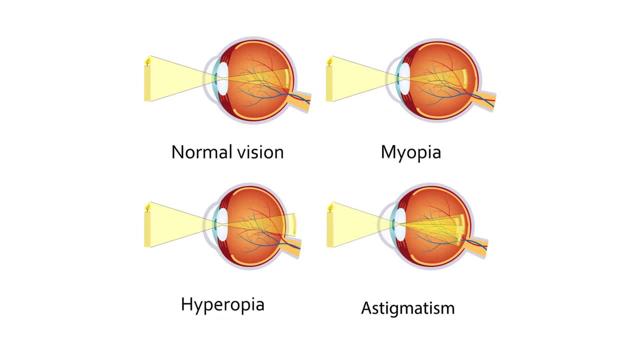 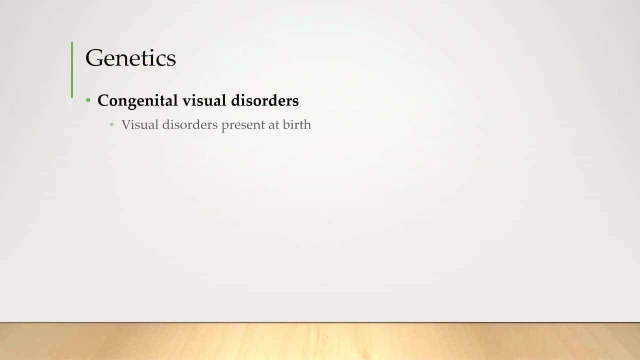 affect the eye. here's a little summary, But for our senior psychology syllabus we don't exactly need to know how this works Now. as well as inherited visual disorders, you can also have congenital visual disorders. That is something that's present at birth. 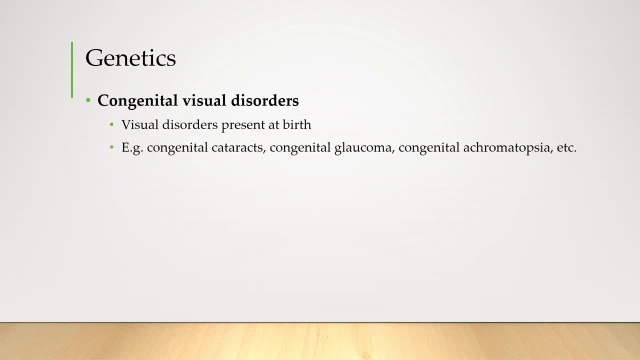 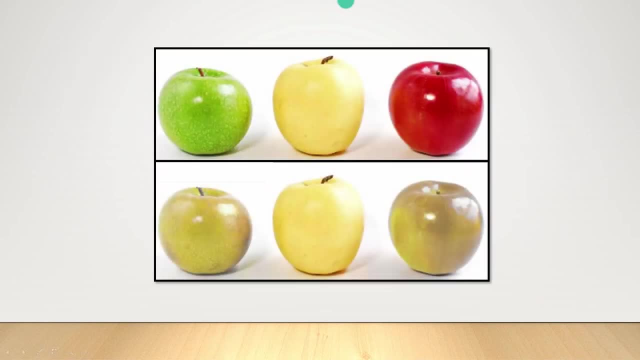 So a few of the things mentioned before, like cataracts, glaucoma, achromatopsia, these can be congenital as well, including one of the most possibly famous visual conditions of all, which is what happens when you see this top image like that. 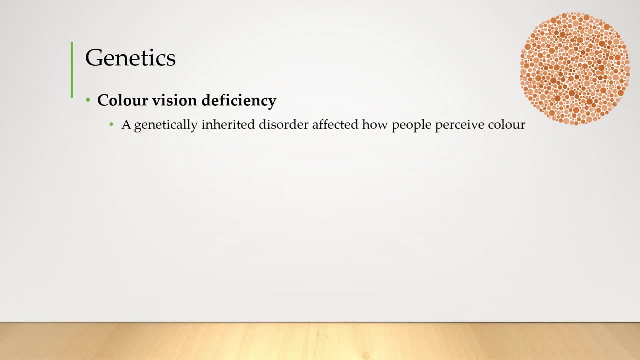 This condition is known as color vision deficiency, which is a genetically inherited disorder that affects how people perceive color. It's also known as color blindness, but that's not really the correct term for it. Color vision deficiency is much more common in men, because this disorder 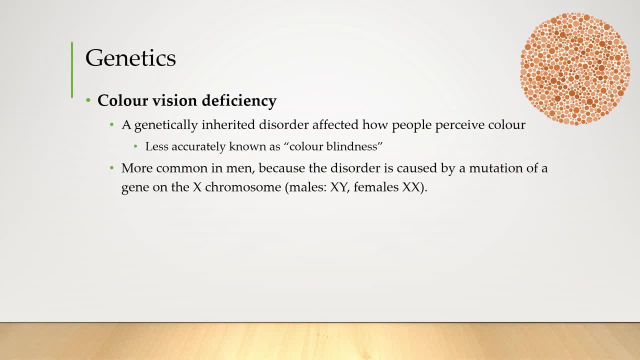 is caused by a mutation of a gene located on the X chromosome. Because females have two X chromosomes- there's sort of a built-in protective factor there- whereas males don't have that. Now. this condition occurs when one or more of the types of cones in the retina